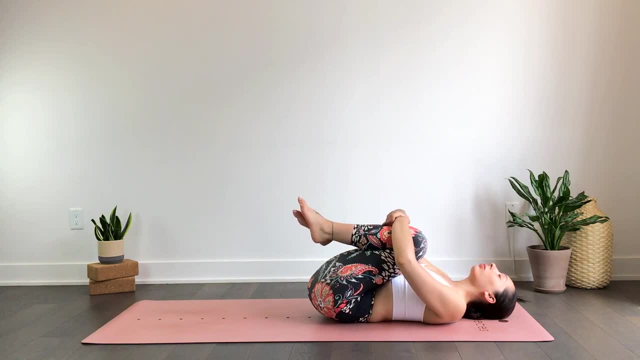 Big hug, big squat, Squeeze, maybe even gently rocking side to side. We'll grab the outer edges of the feet, bottoms of feet, to touch. You can stay right here or rock side to side. Okay, Now, on your next inhale you can come up to a tabletop pose or you can. 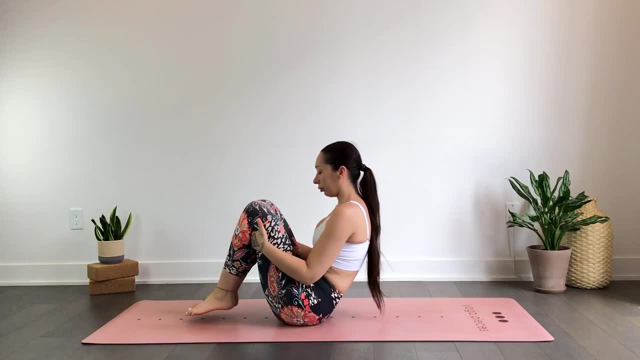 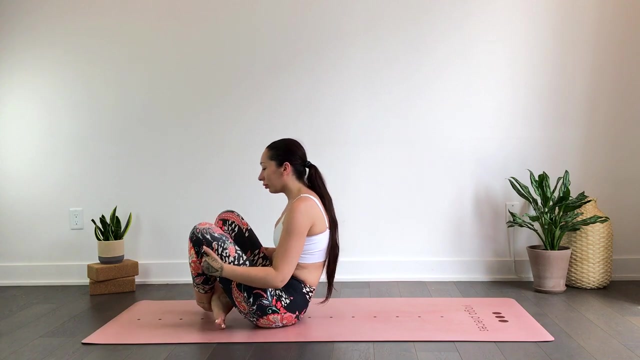 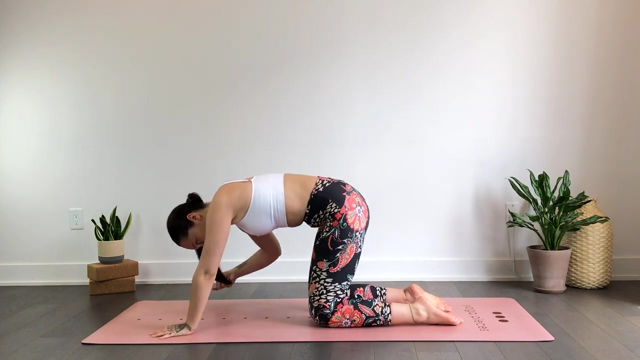 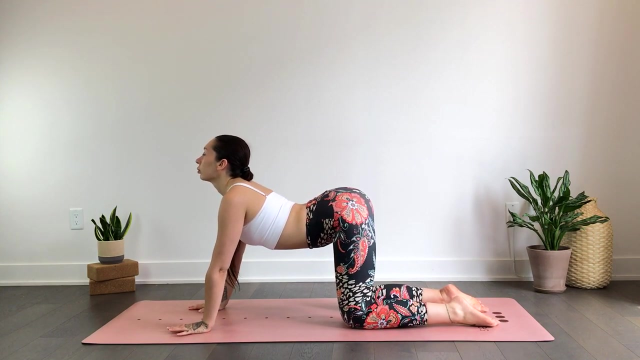 gently rock forward and back, tucking the chin, protecting the neck. and when you're all ready, we'll come to a tabletop. pose wrists under shoulders, knees under hips, inhale, dropping the belly. take your gaze up for cow pose, exhale, rounding through the spine. take your gaze down for cat, and you can. 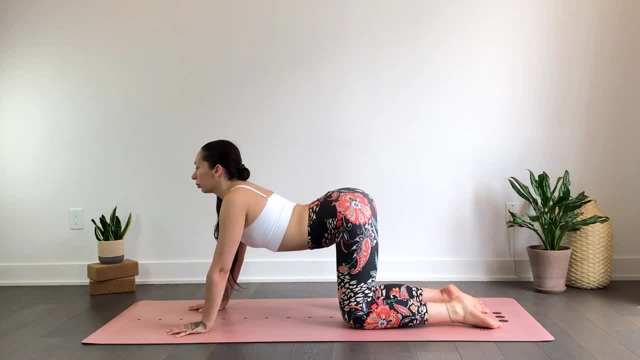 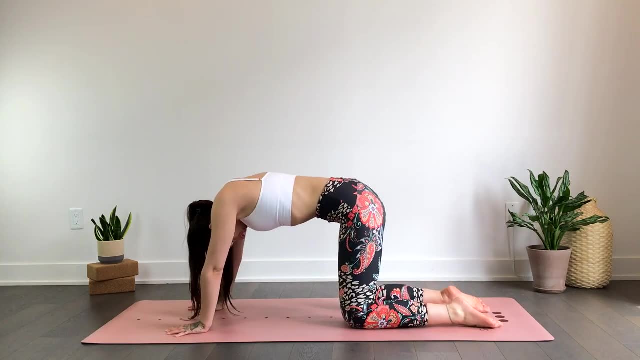 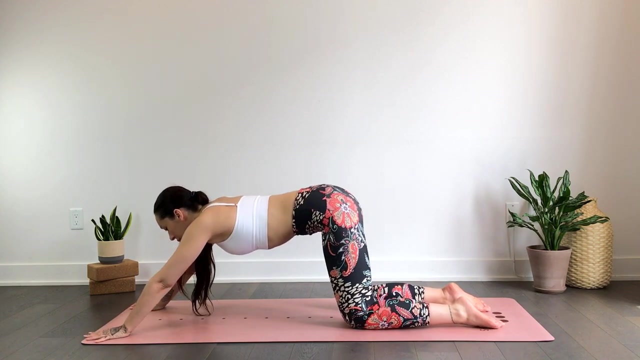 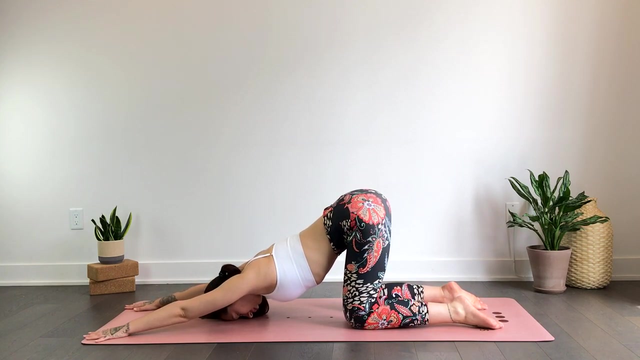 continue sinking breath with movement, or you can even find some organic movement if that feels better. today, we'll come to a neutral spine, walking the hands towards the top of the mat, keeping the hips over the knees as you melt the forehead down towards the mat or resting it on a block. now, if it's available today, feel free to take the. 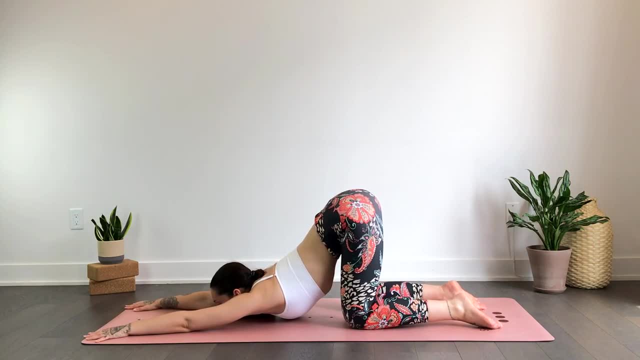 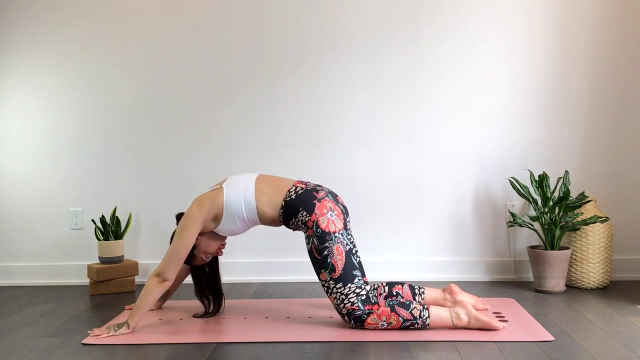 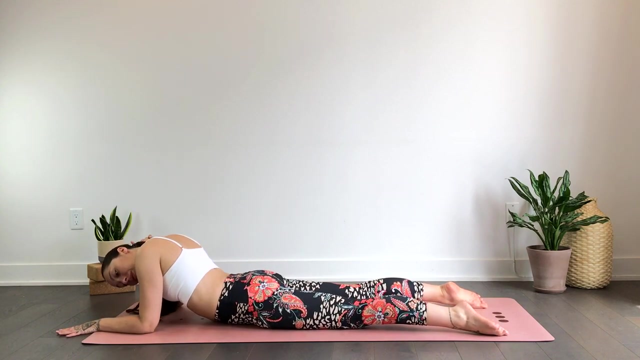 chin and chest to the mat, staying wherever you feel most comfortable, focusing on the breath, observing the body on your next inhale, rounding through the spine all the way down to your belly, resting on your forearms, tucking the tailbone, pressing the pubic bone into. 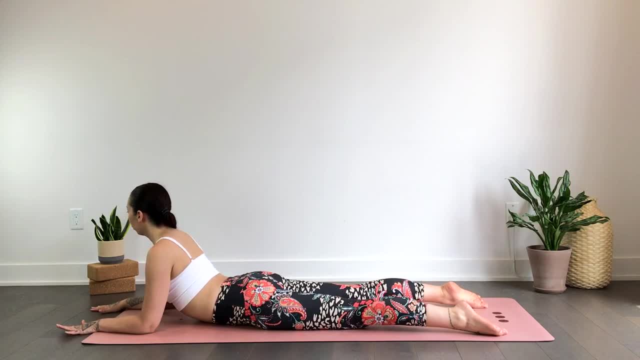 the mat. inhale as you lift through the sternum. exhale, softening the shoulders. take a moment here to observe the belly pressing into the mat as you inhale. softening the belly as you exhale. we'll release planting the hands underneath the shoulders, tucking the 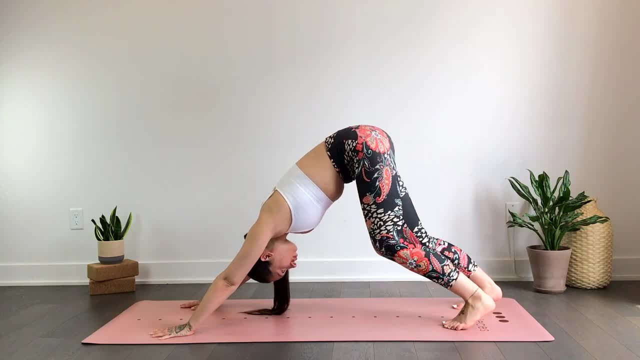 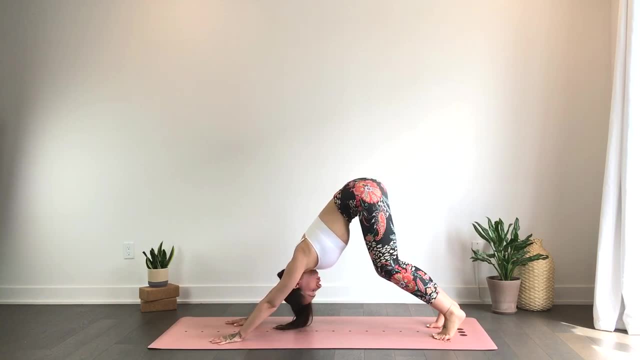 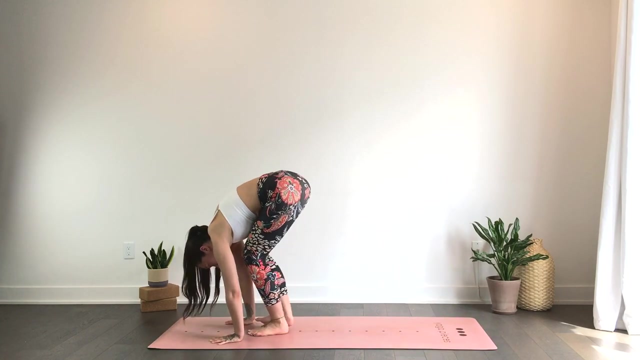 toes. use a bit of your core here, sending the hips up for down dog. feel free to walk it out. bending one knee, bend the other, pressing the mat away from your hands and feet: inhale, stepping to the top of the mat, coming right into a half lift flat back. 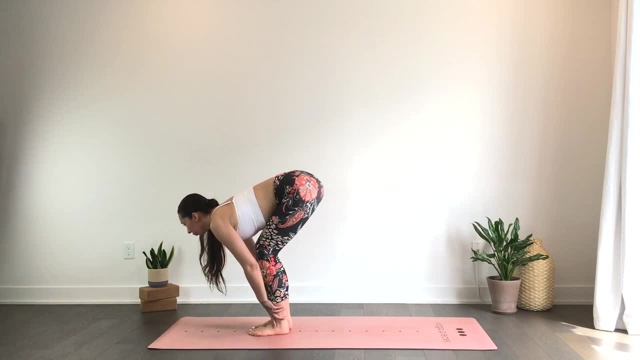 come up as high as you need- exhale- bending the knees. take a fold- inhale. come to standing hands. reach up. exhale- heart center. inhale the hands. reach up. exhale. take a fold option to bend the knees. exhale. take a fold option to bend the knees. 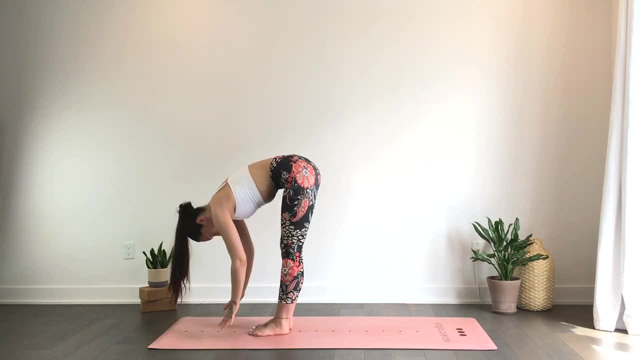 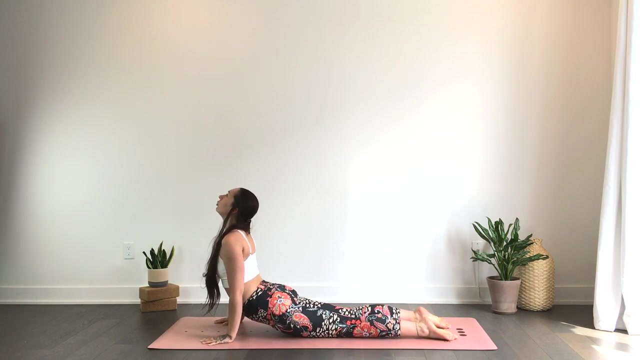 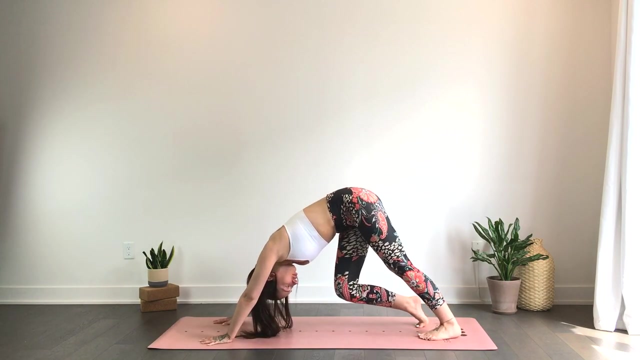 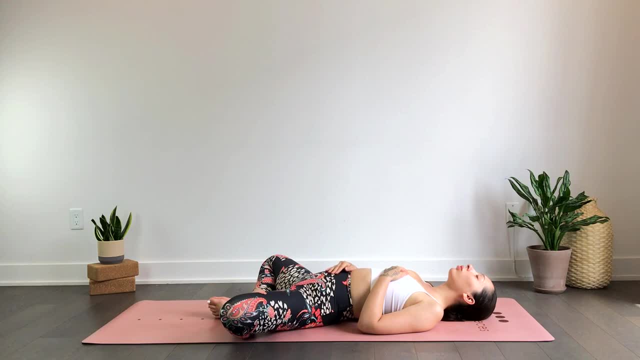 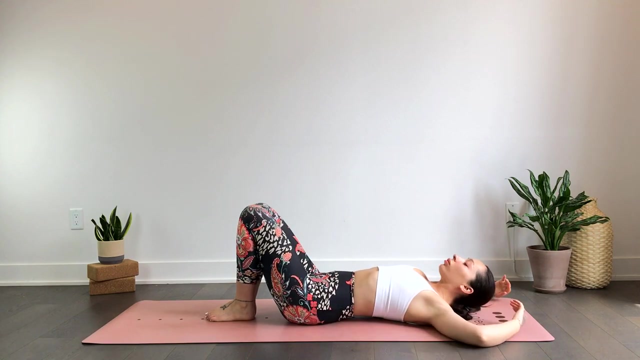 exhale: tuck the toes, sending the hips up for down. dog walk it out here, maybe bending both knees, bending one, bend the other. inhale lifting the knees. inhale: lifting the knees. inhale: lifting the knees as you exhale, taking both knees over as you exhale, taking both knees over. 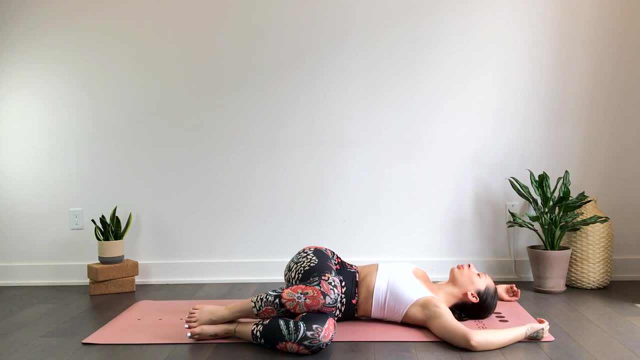 as you exhale, taking both knees over towards the left back stays flat on the towards the left back stays flat on the towards the left back stays flat on the mat mat. mat for a supine twist for a supine twist, for a supine twist option here to place pillows between the 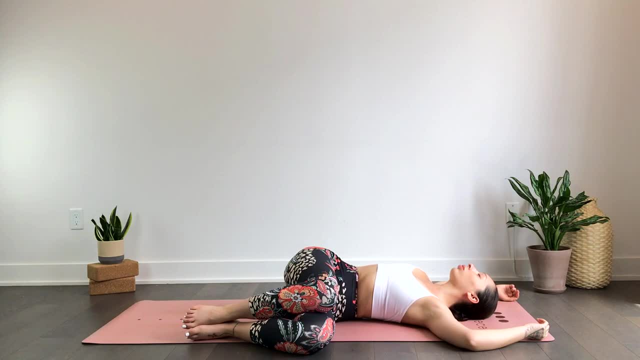 option here to place pillows between. the option here to place pillows between the knees and underneath the knees for added knees and underneath the knees for added knees and underneath the knees for added height and support. height and support, height and support. you can even place a pillow underneath. 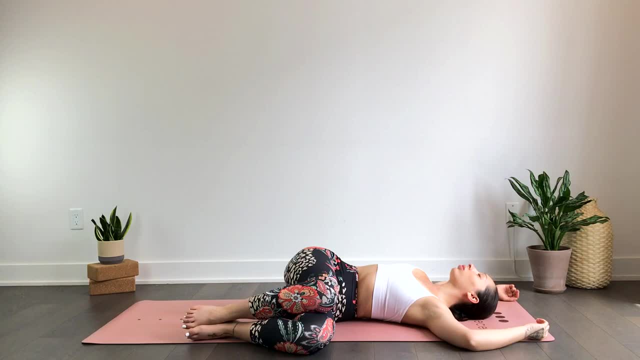 you can even place a pillow underneath. you can even place a pillow underneath the right shoulder for added height. less the right shoulder for added height, less the right shoulder for added height. less of a twist, trying the breath into the belly and trying the breath into the belly, and 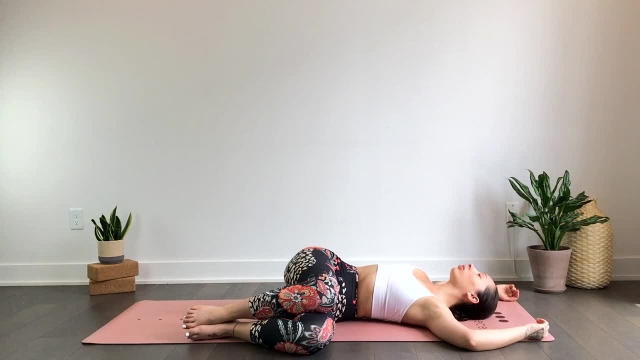 trying the breath into the belly and softening the belly, softening the belly, softening the belly with each exhale, with each exhale, with each exhale. inhale to lift the knees. exhale will inhale to lift the knees. exhale will inhale to lift the knees. exhale will take them over towards the right again. 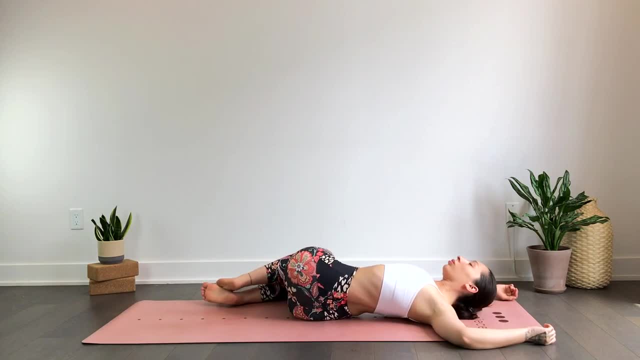 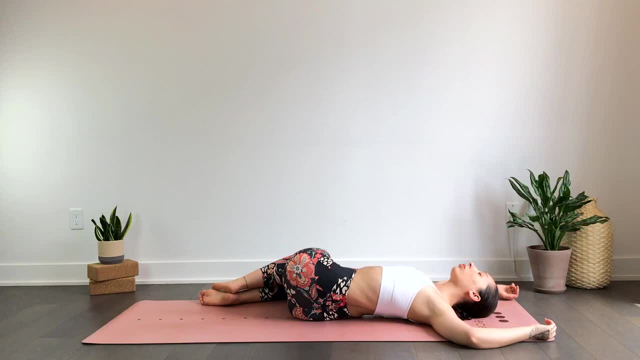 option to modify if needed. option to modify if needed. option to modify if needed. and will gently lift the knees, take the. and will gently lift the knees, take the. and will gently lift the knees, take the. feet mat with distance and just gently. feet mat with distance and just gently. 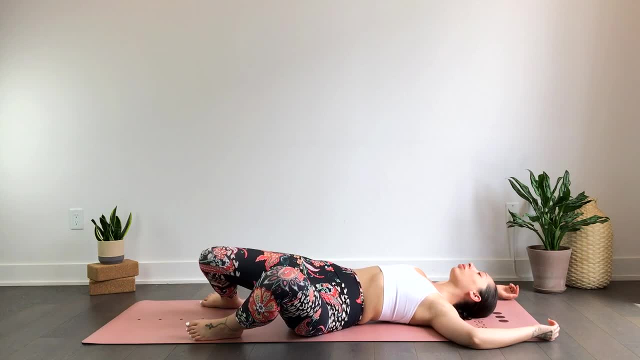 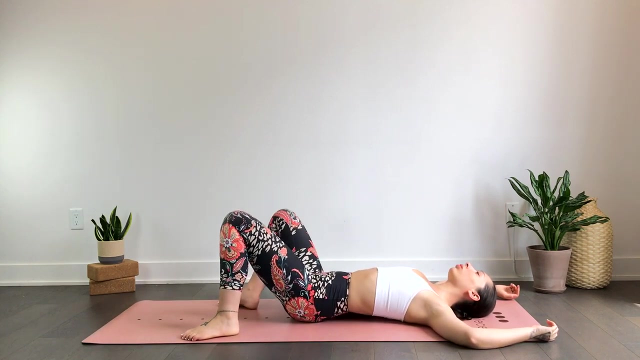 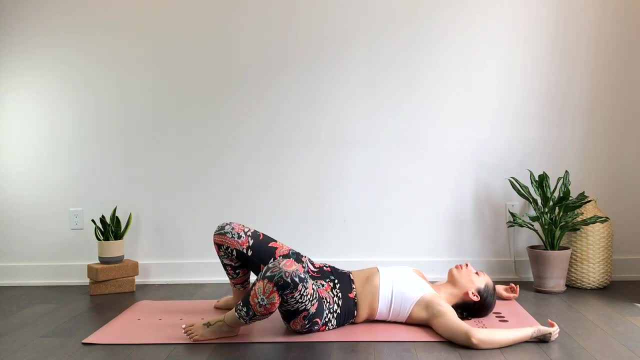 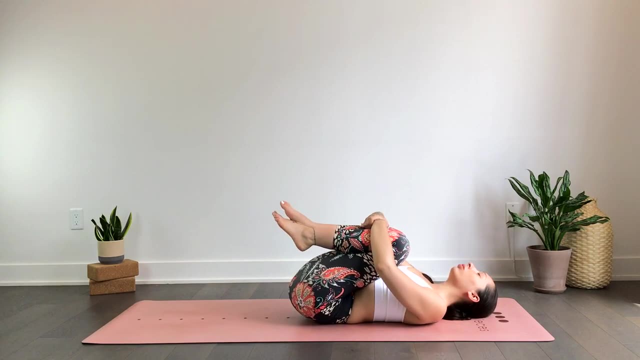 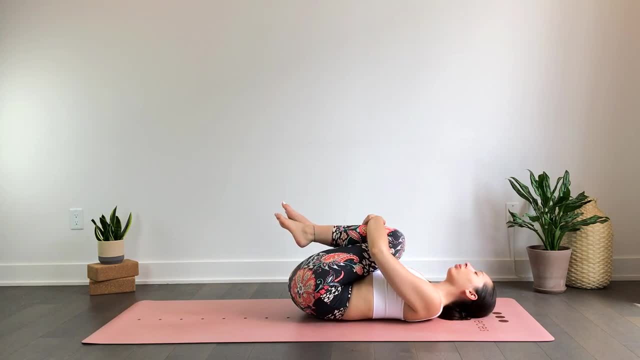 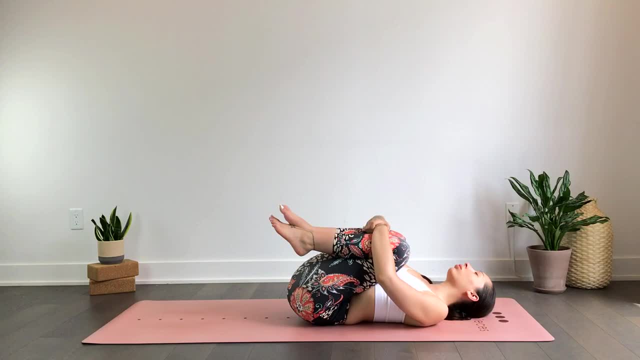 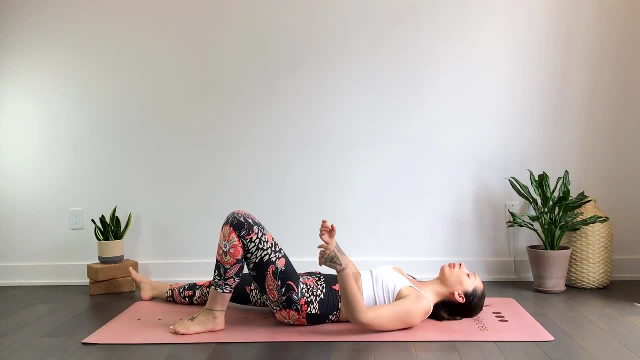 shavasana, taking the shavasana, taking the feet to the bottom of the mat, hands to feet to the bottom of the mat, hands to feet to the bottom of the mat, hands to your sides, palms facing up, taking this one moment out of our 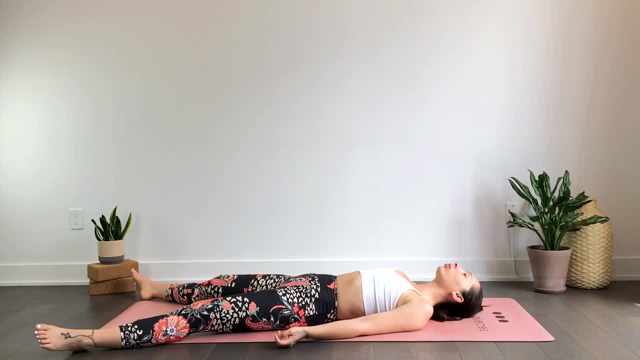 taking this one moment out of our, taking this one moment out of our practice, practice, practice out of our day, sometimes out of our week, out of our day, sometimes out of our week. out of our day, sometimes out of our week, to just be, to just be, to just be, to be here with the body in its fully. 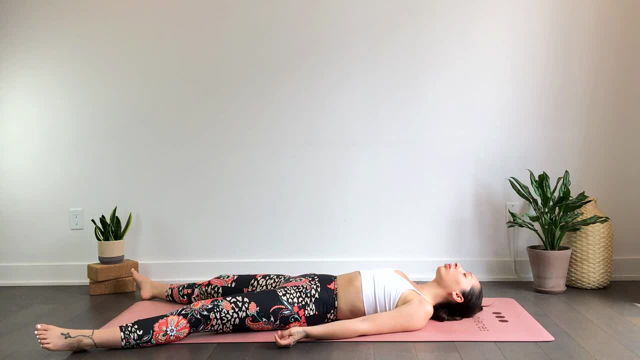 to be here with the body in its fully. to be here with the body in its fully, relaxed and present state, relaxed and present state, relaxed and present state, to soak in all the work we just did and to soak in all the work we just did and to soak in all the work we just did and to give gratitude. 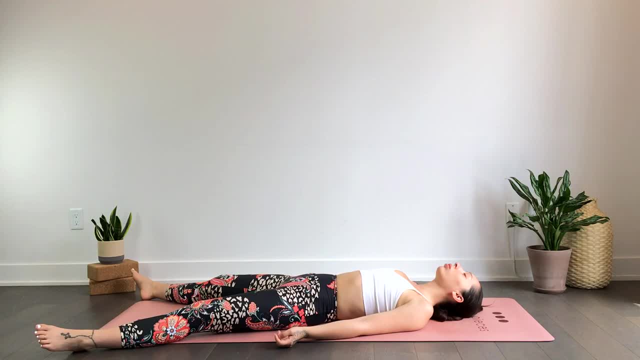 to give gratitude. to give gratitude to ourselves for showing up to the mat. to ourselves for showing up to the mat. to ourselves for showing up to the mat. know that you are worthy of this time. know that you are worthy of this time. know that you are worthy of this time and the space is here for you any time. 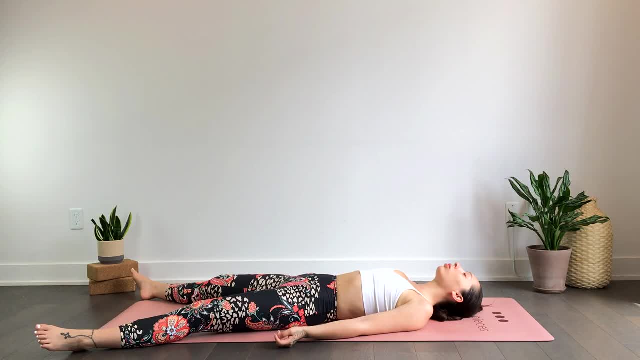 and the space is here for you any time and the space is here for you any time that you need that. you need that you need. we'll rest here a few moments. we'll rest here a few moments. we'll rest here a few moments. Let's pray. 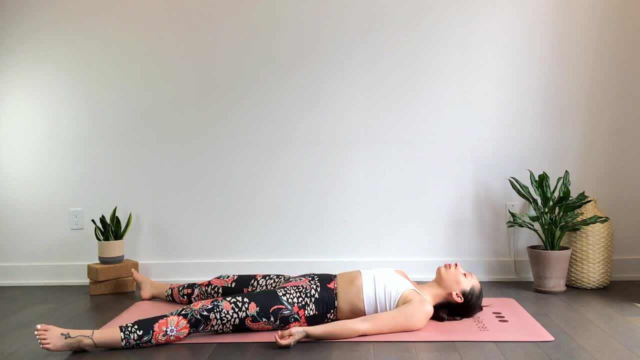 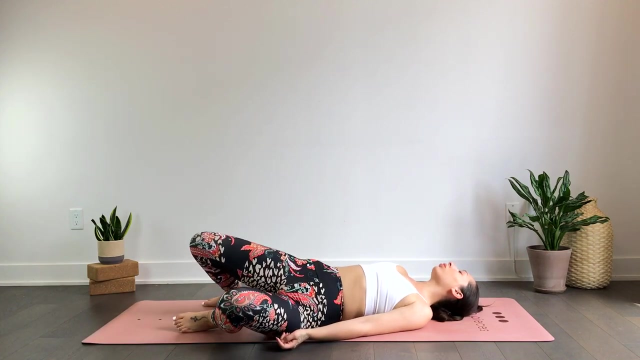 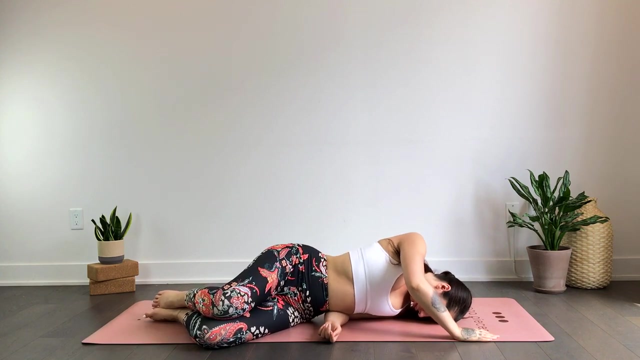 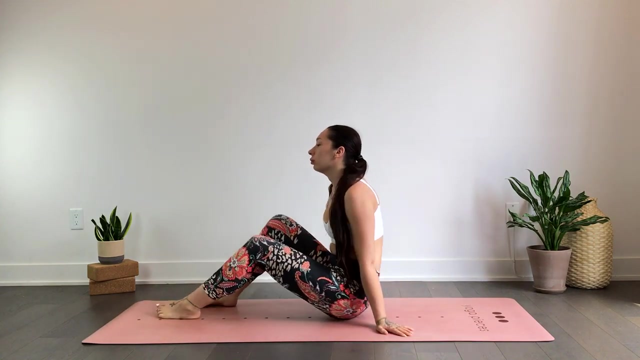 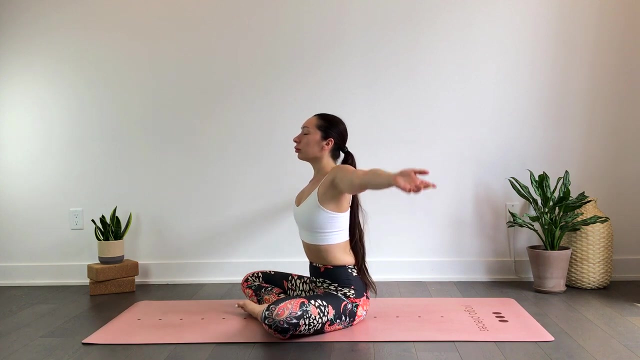 We'll gently begin to wake up the body wiggling the fingers and toes, rocking the head side to side. We'll roll over towards our right full inhale and exhale, coming to a comfortable seat. We'll inhale the hands up overhead, exhale heart center.